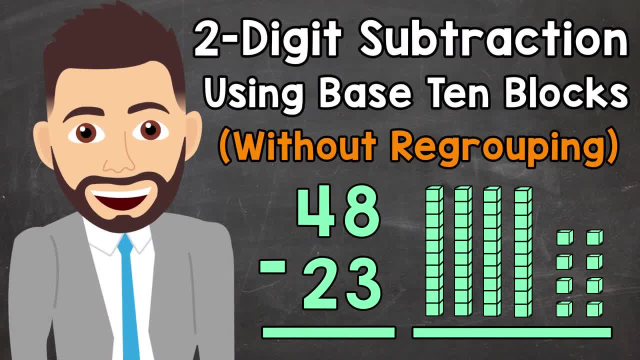 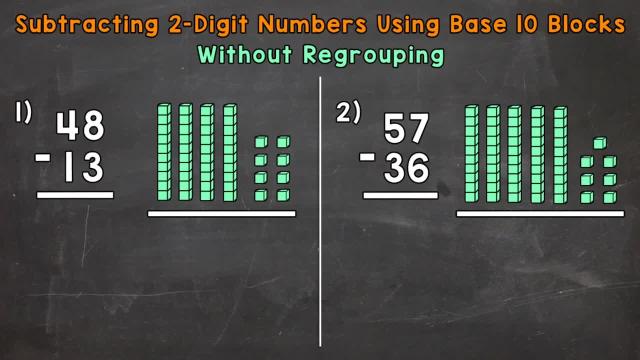 Welcome to Math with Mr J. In this video, I'm going to cover how to subtract two-digit numbers using base 10 blocks. These problems are going to be without regrouping or borrowing. Now, using base 10 blocks is going to help us visualize and better understand subtraction. So let's jump into. 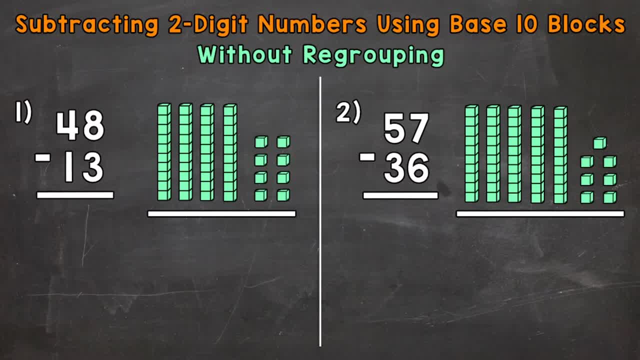 number one, where we have 48 minus 13.. So we're starting with 48 and subtracting or taking away 13.. To the right of the problem, I have 48 represented by base 10 blocks. So the number 48 has a 4 in the tens. place This 4 right here. That 4 represents four tens and has a value of 40.. 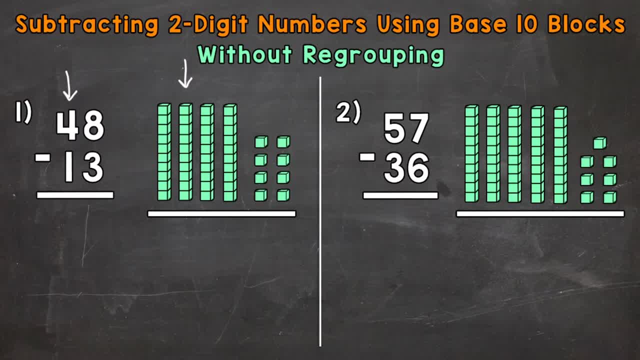 So here are our four tens. Now, in the ones place we have an 8. That 8 represents eight ones and has a value of 8.. So here are our eight ones. So now we need to subtract or take away 13.. Now, when we subtract, 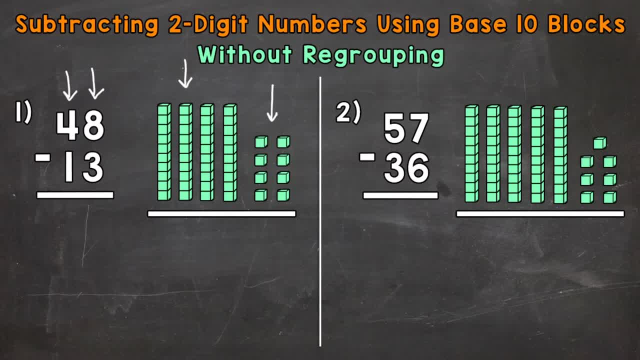 whole numbers. we start with the ones place, So eight ones minus three ones. So let's subtract or take away three from the eight, So eight times in the tens place we have a total of one and that wn. So again that will be one, three, eight. 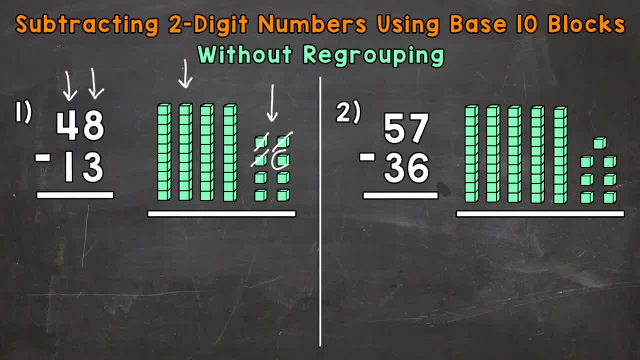 Let's try to tracks this point. Let's get things going on and now let's move on to the tens place. Before we move on to our tens place- our tens place- we will want to Take legal due back. So our tens place should say 10 plus. four, 10 to the tens place. So again we're going to subtract or take away your tens. So we need to subtract or take away One, two and three. Now you can see how many we have left: One, two, three, four and five. So five goes into one's place in our answer. 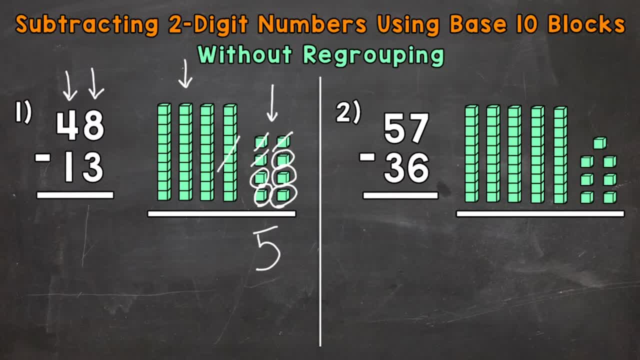 Which one is one. So we have four tens minus one-tens minus one-tens. So we need to subtract or take away 13 at schoolwork, away 110.. 1. Now we need to see how many tens we have left. So we have 1,, 2, and 3.. 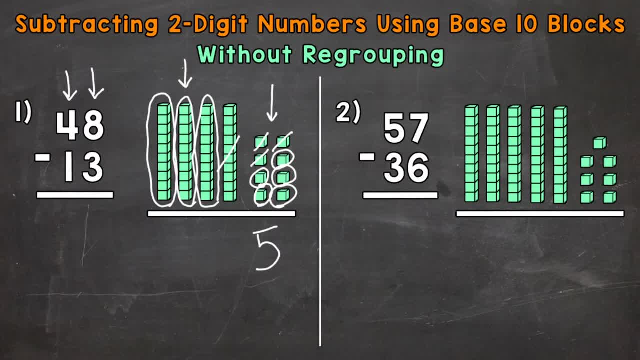 So we put a 3 in the tens place in our answer. So our answer is 35. Let's go to the left, to the original problem, and subtract there as well to see if we still get 35. Again, we start with the ones. So 8 minus 3, that gives us 5.. And 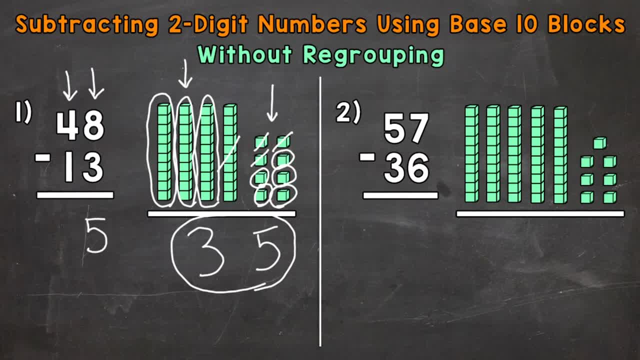 then, as far as the tens- 4 minus 1, that gives us 3. So we have 35 over there as well. Let's move on to number 2, where we have 57 minus 36.. So we have 57. 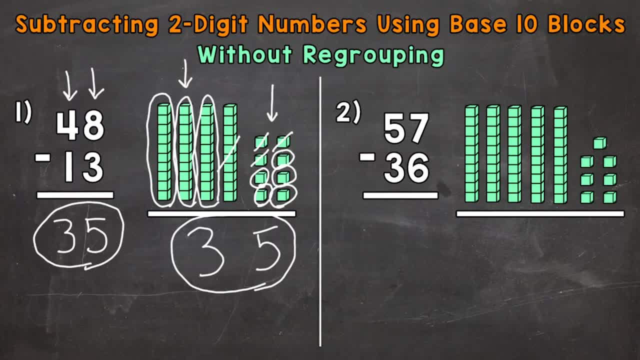 represented by the base 10 blocks to the right. 57 has a 5 in the tens place. So 5 tens right here and then a 7 in the ones, So we have 7 ones right here. Let's start by subtracting the ones, So we have 7 ones minus 6 ones. So let's. 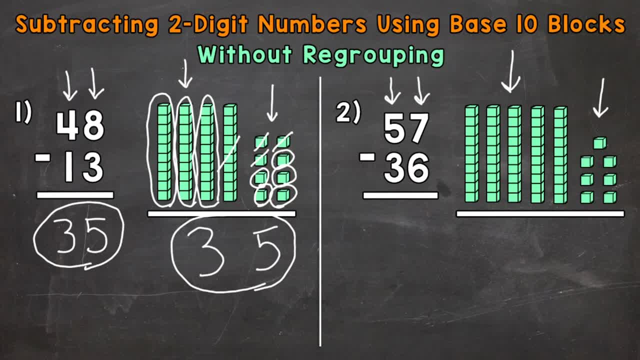 take away or subtract 6 from the 7.. 1,, 2,, 3,, 4,, 5, 6.How many do we have left? Well, 1.. So 1 goes in the ones place in our answer. 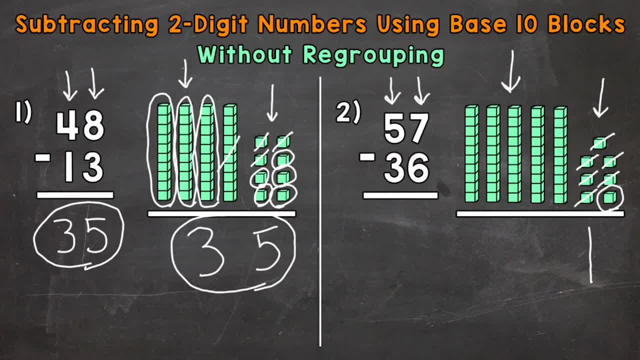 Now for the tens. So we have 5 tens minus 3 tens. So let's take away or subtract 3 tens, 1, 2, 3.. How many do we have left? 1, 2.. So we put a 2 in the tens place in our answer and we get an answer of 21.. 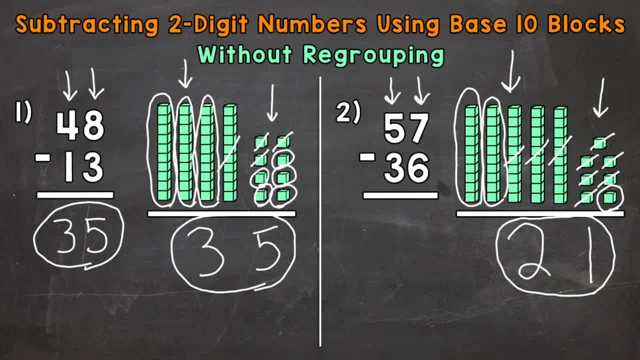 Let's solve the problem to the left as well and see if we still get 21.. Start with the ones: 7 minus 6 equals 1.. Now for the tens: 5 minus 3, that equals 2.. And we get 21 over there. 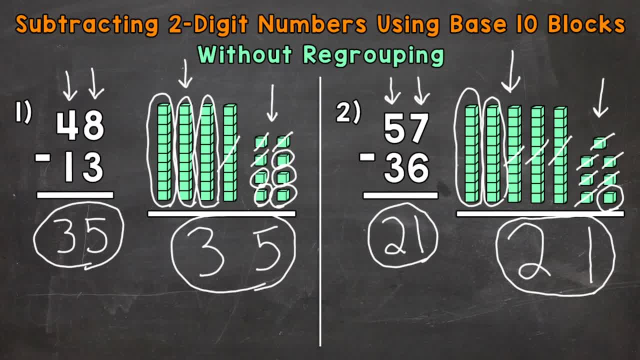 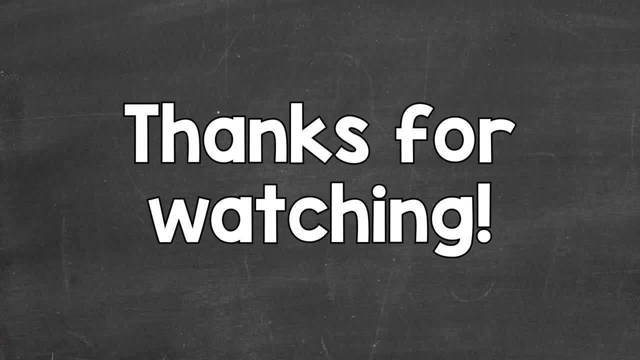 As well. So there you have it. There's how you subtract two digit numbers using base 10 blocks. I hope that helped. Thanks so much for watching. Until next time, peace.